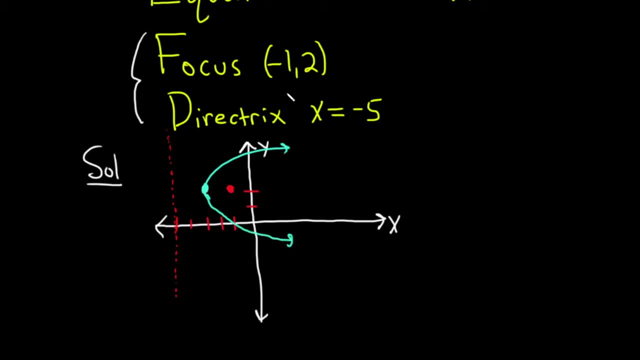 we'll just assume it is Okay. so now we can write down the formula Because it opens, right? we know that the y is being squared, So parabolas that open up and down have the x being squared. Parabolas that open left or right have the y being squared, So parabolas that open up and down have the 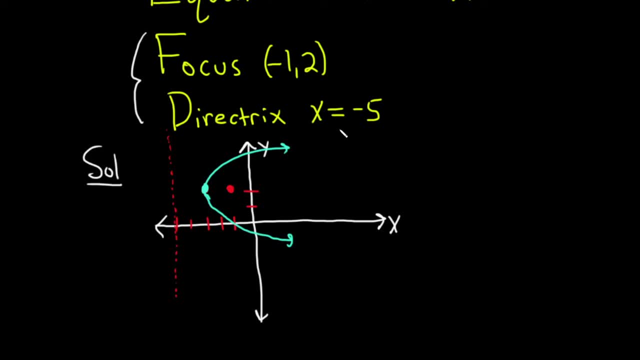 y being squared. So if it opens up or down, the x is squared. If it opens left or right, the y is squared. So the formula is: y minus k squared equals 4c, x minus h. If it had opened up or perhaps down, the formula would have been: x minus h squared equals 4c, y minus. 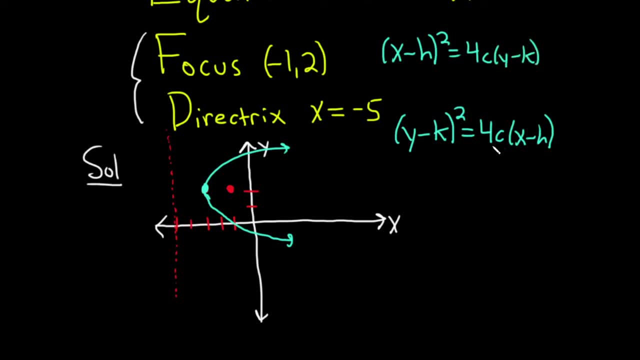 k. So the thing is that the x always goes with the h and the y always goes with the k. It's just a trick to remember it. Okay, so now all we have to do is plug stuff in, So the vertex here. let's just write it down as an ordered pair. It looks like it's. 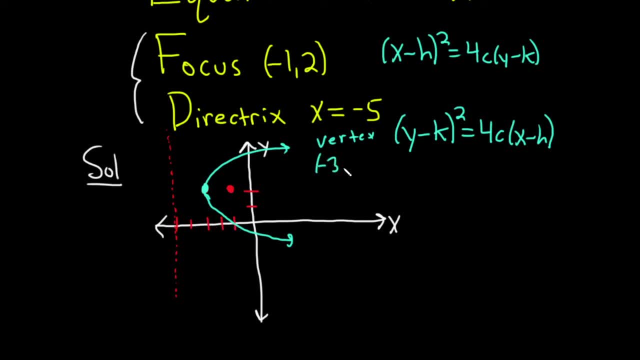 1, 2, 3, 1, 2.. It's negative 3 comma 2.. So this is the h and this is the k, right. So 1, 2,, 3, 1, 2.. So it'll be y minus 2. quantity squared, just like that, equals 4c x plus 3. It's a plus. 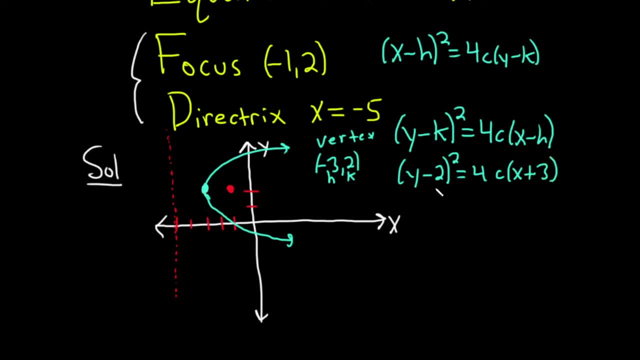 3, because there's already a minus there from the negative 3. And so negative and negative is positive. Alrighty, so now we just have to find c. So the absolute value of c is this distance here, Which we see that it is 2.. Now, because it opens right, c is positive. So c is equal to 2.. If it 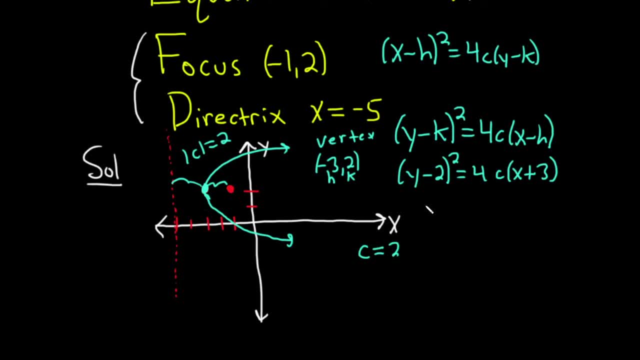 had opened left c would be negative 2.. So this becomes: y minus 2 squared equals 4 times 2 x plus 3. Just replacing the c there with 2.. And so the final answer would be y minus 2 squared. 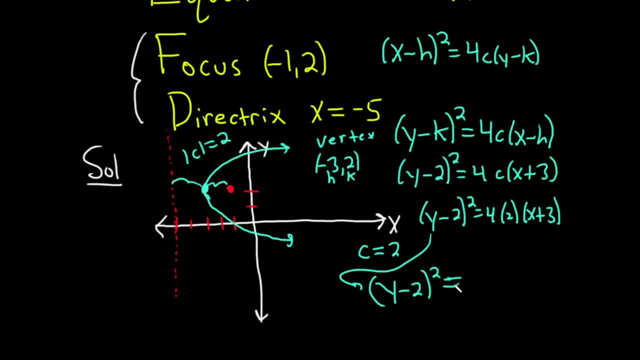 x plus 3.. Equals 4 times 2 is 8.. So this is 8 parentheses x plus 3. And that would be the final answer. I hope this video has been helpful. Good luck.